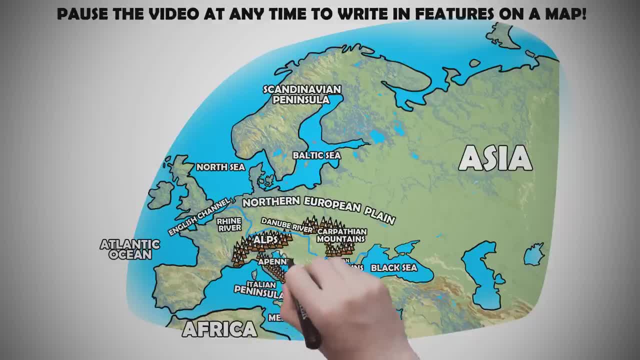 The Apennine Mountains span the majority of the Italian Peninsula. The last major mountain range in southern Europe are the Pyrenees, which separated mainland Europe from the Iberian Peninsula, where modern-day Spain and Portugal reside. The Strait of Gibraltar is a narrow body dividing Spain with Morocco. 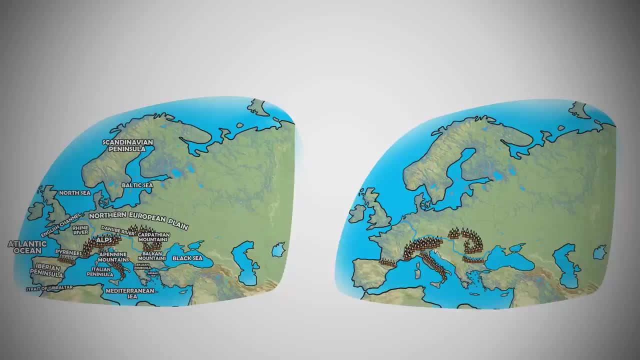 Test your knowledge. Let's play Follow the Fish. In this game, you will track the fish as it appears on a blank map of Europe. Once the music stops, you will use a map of Europe labeled with physical features to determine where the fish ended up. 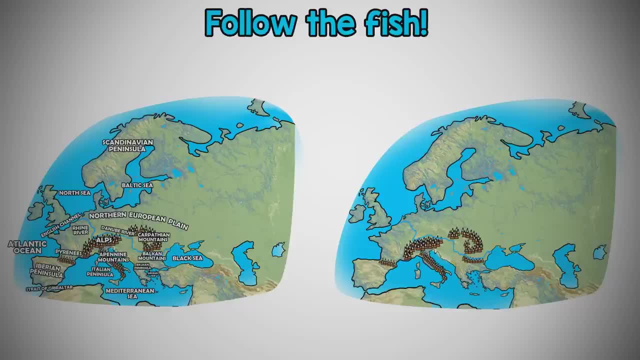 Other animals may appear on the map, so don't forget to keep your eyes on the fish. Follow the Fish, Follow the Fish. So where did the fish end up? Was it the Alps, the Balkan Peninsula or the Black Sea? That's right, It was the Balkan Peninsula. 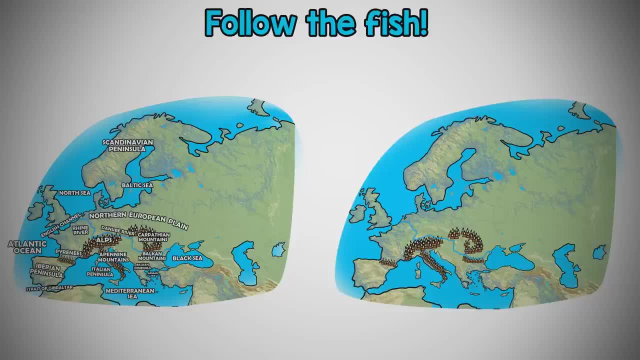 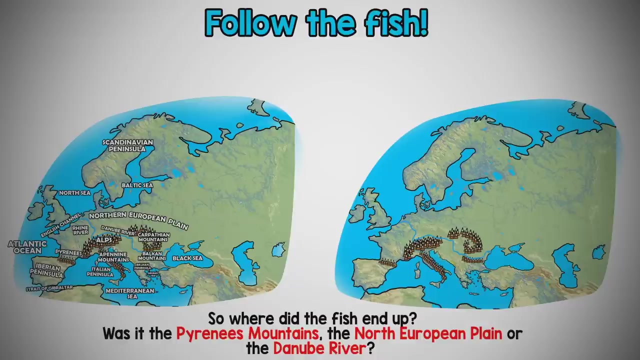 Let's try it again. Remember to keep your eyes on the fish, Follow the Fish. So where did the fish end up? Was it the Pyrenees Mountains, the North European Plain or the Danube River? Yep, it was the Danube River. 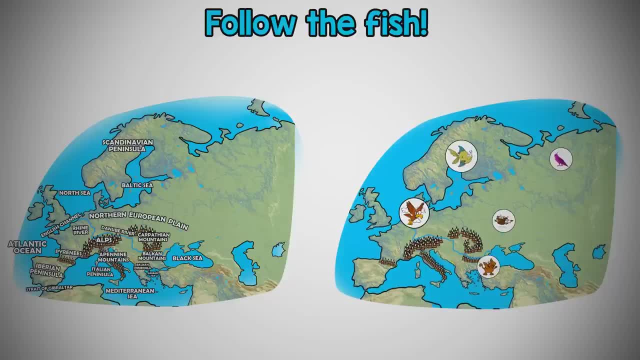 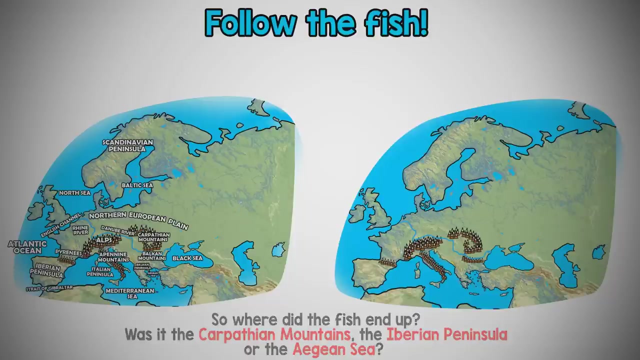 Let's try one last time. You got this. So where did the fish end up? Was it the Carpathian Mountains, the Iberian Peninsula or the Aegean Sea? Nice job, It was the Carpathian Mountains. 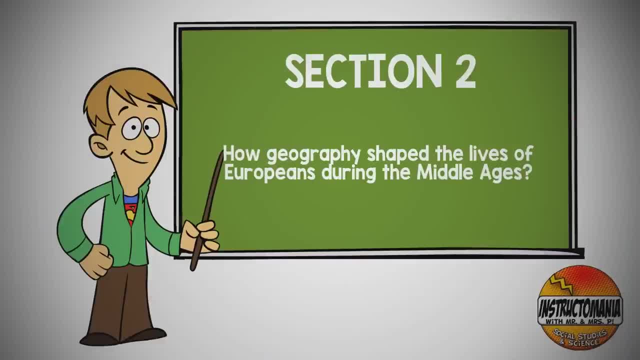 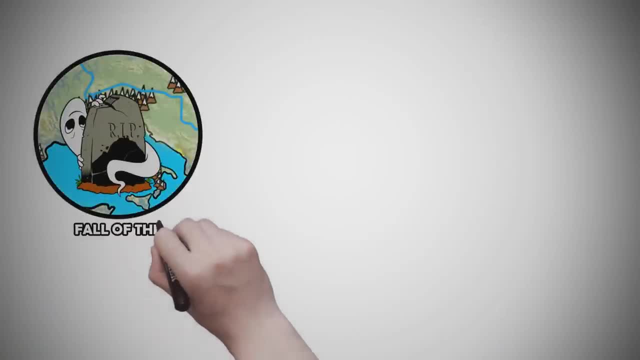 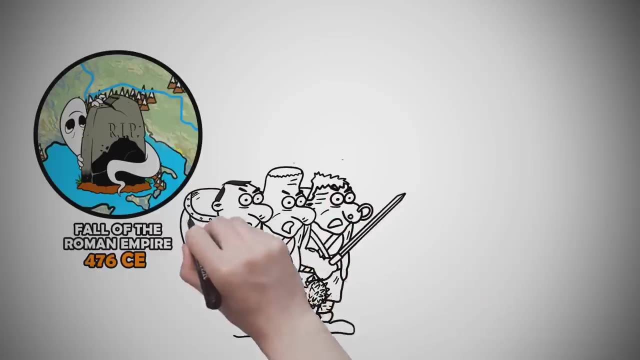 How geography shaped the lives of fish, The lives of Europeans, during the Middle Ages. The Middle Ages, also known as the Dark Ages, started after the fall of the Roman Empire in 476 CE, Because of the lack of protection from the former Roman Empire. 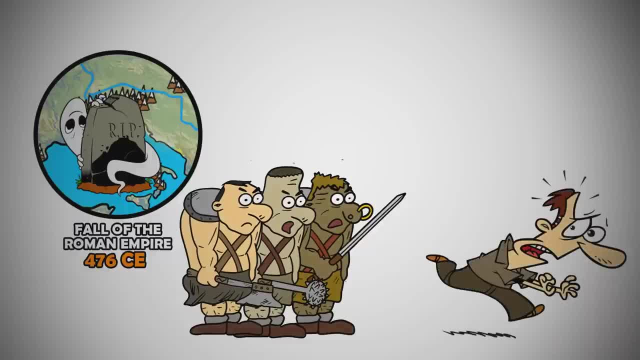 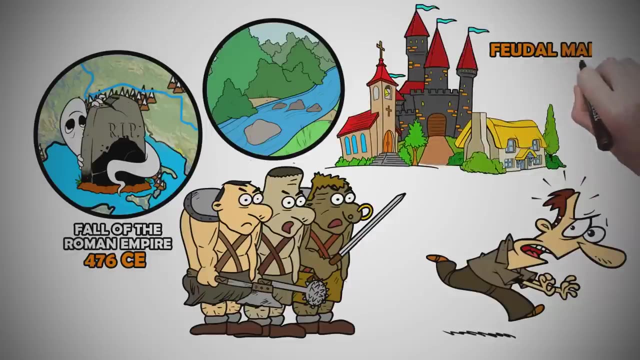 people had to look elsewhere for protection from often barbaric groups competing over resources. Groups of people battled for control of different regions, especially those with freshwater rivers for agriculture and food supply. Feudal manors that offered a system of protection from invaders popped up along water sources and trade routes. 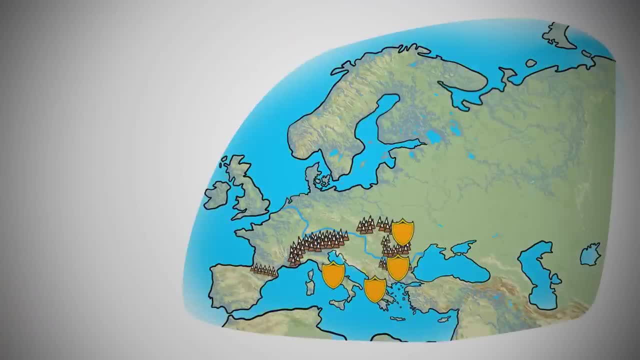 The many mountain ranges in the southern regions of Europe created a barrier of protection from Arabian, Asian and African invaders. However, the flatland of the Great European Plain and the deep waters of rivers such as the Danube allowed northern invaders deep into Europe. 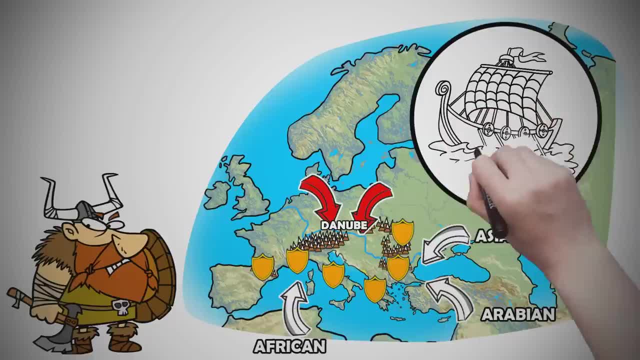 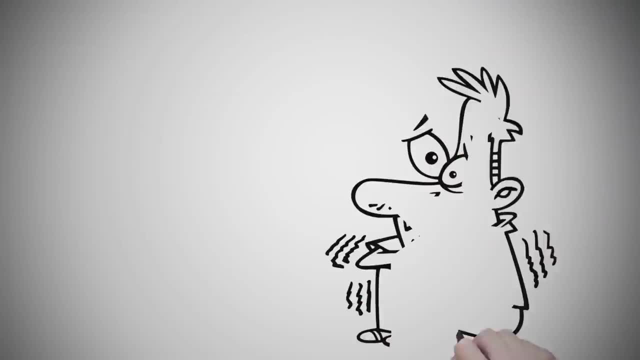 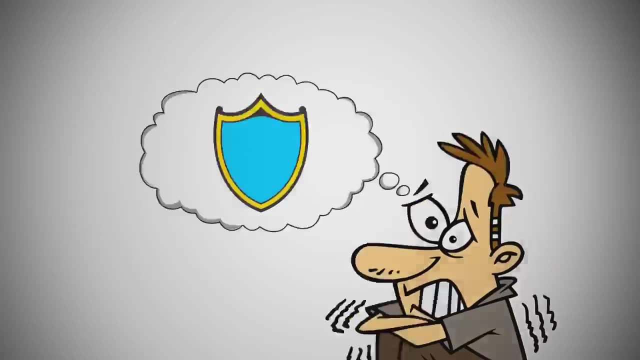 Vikings in particular used narrow ships called the Danube. Phoenicians in particular used long ships, called the long ship, to move swiftly down rivers and into European countrysides to attack quickly. The constant fear of attack meant that people were willing to sacrifice freedom for a localized system of protection. 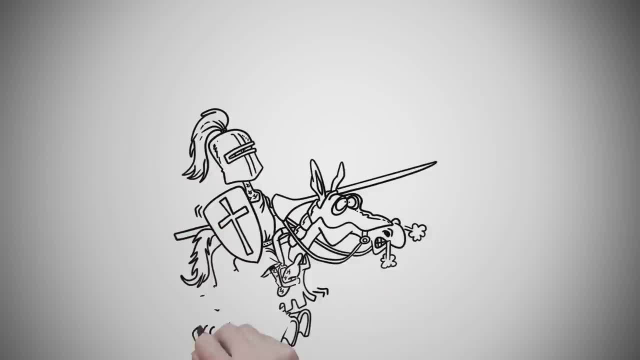 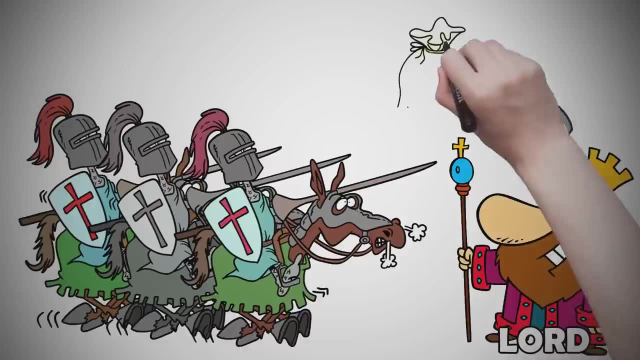 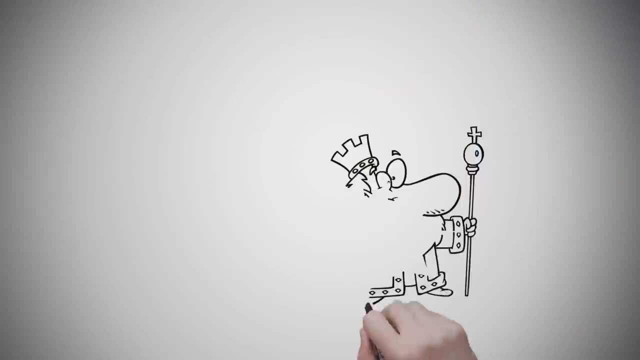 Who lived in medieval Europe. In order to protect their land and people, European lords created and trained their own armies. Often, these armies included knights, men who were paid in money and land to swear allegiance to their lord and fight for him. Lords and their families lived in luxury and oversaw their agricultural and trade interests. 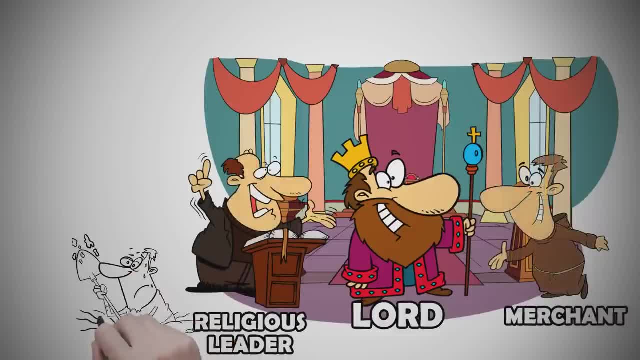 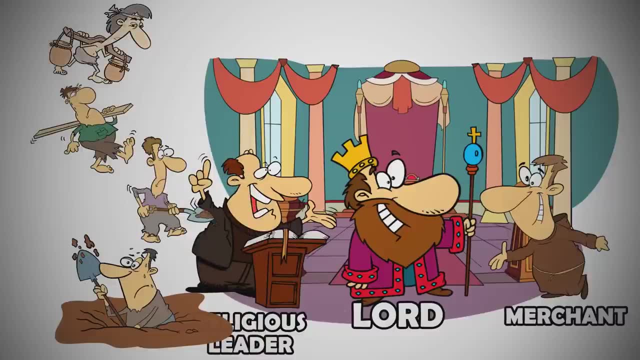 They often did business with merchants and religious leaders. Peasants, referred to as serfs, lived, worked and often died in the service of their lord. Whole families and generations of serfs continued to work and live on the same lord's land or in his household. 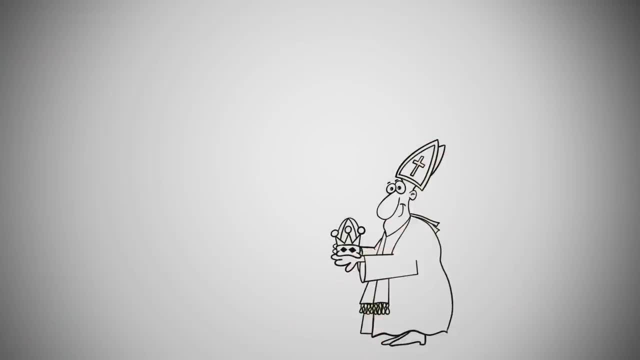 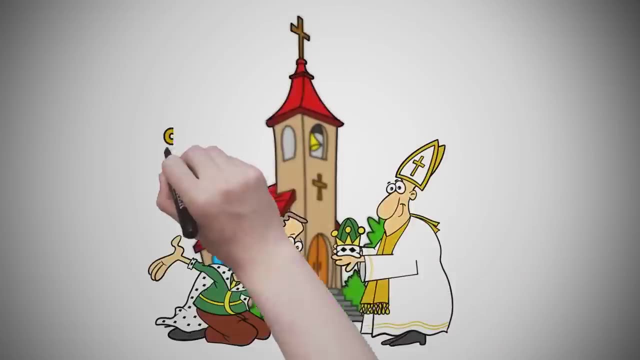 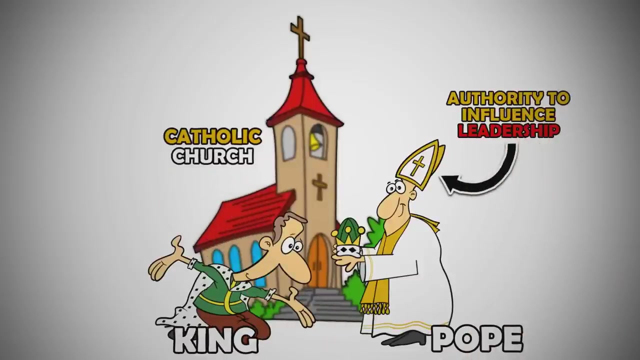 Religion played an important role in feudal European society. Catholic Christianity dominated, In fact. as the leader of the Catholic Church, the pope even crowned the king of the Holy Roman Empire, giving the pope ultimate authority to influence leadership. Manners had their own church buildings and a resident priest, bishop or deacon. 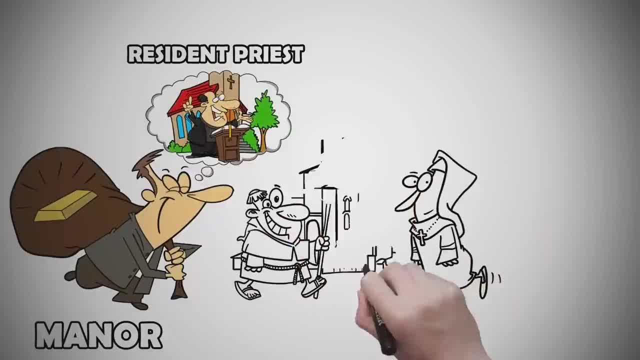 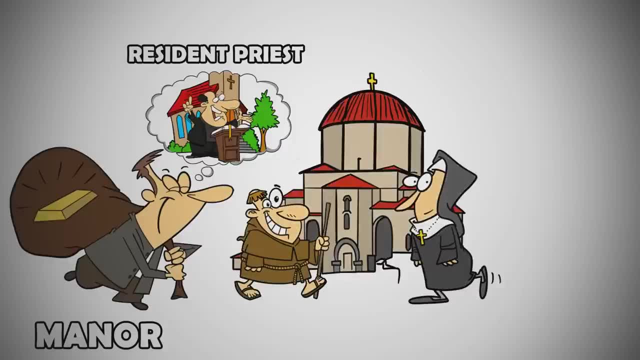 Monasteries and nunneries also sprang up in medieval Europe, where groups of men or women decided to live separately from the rest of society in service to God and their fellow men. Poor monks, called friars, traveled and served as needed in exchange for food and basic necessities.